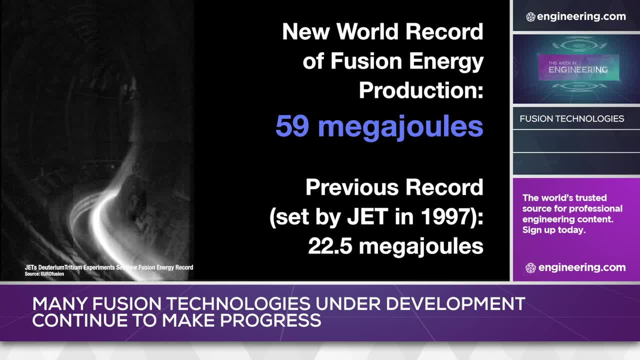 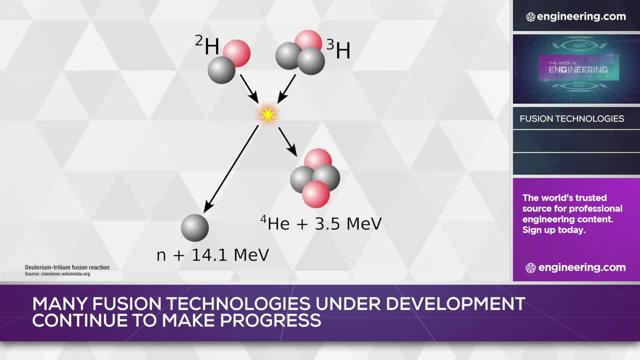 of water, but it surpasses the previous record from 1997, when 22 megajoules of heat were produced. The reaction burned a deuterium and tritium fuel mix, the same fuel currently used in the much larger ITER tokamak in southern France, and the JET team expects that their progress in stable plasma 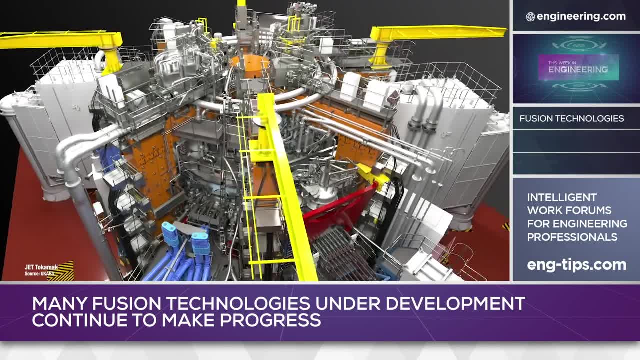 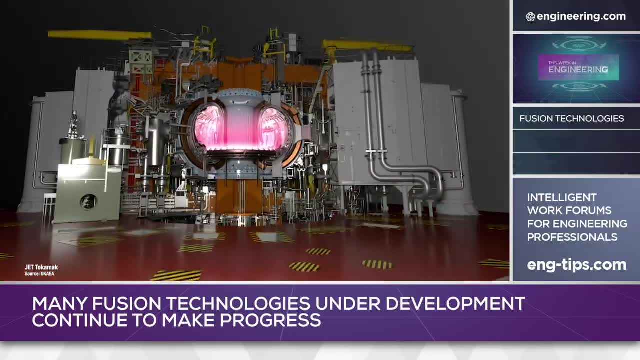 containment will have applications in the much larger project. Both JET and ITER are toroids and use magnetic confinement to contain the super hot plasma. For decades this was considered the only practical way to handle plasma which is so hot that no known material can contain it. There are 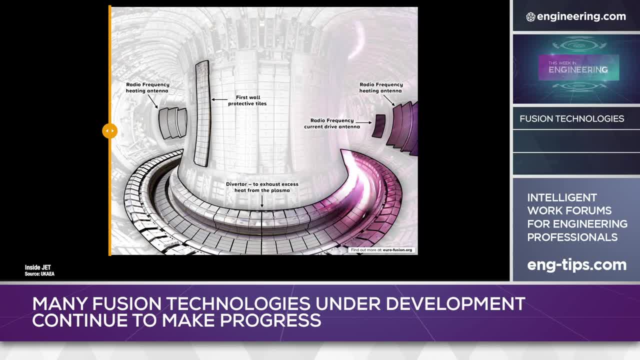 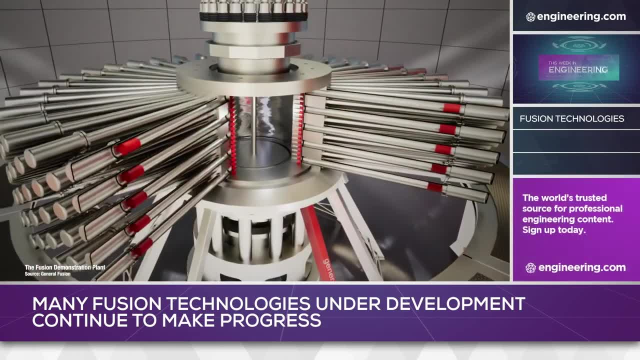 other alternate techniques, one of which is under construction now by Vancouver, Canada-based General Fusion. The firm uses a unique technique- mechanical compression of a large spherical mass of liquid metal to symmetrically collapse a liquid vortex cavity in a few milliseconds. The fusion reactions 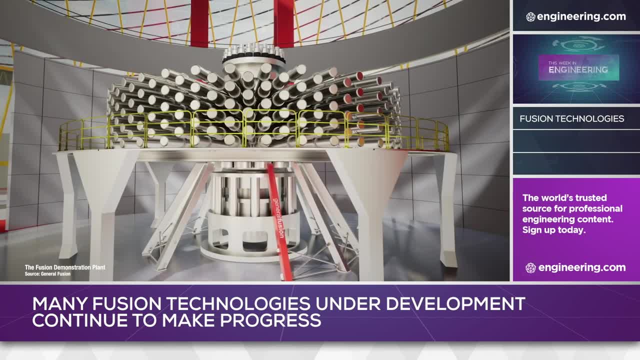 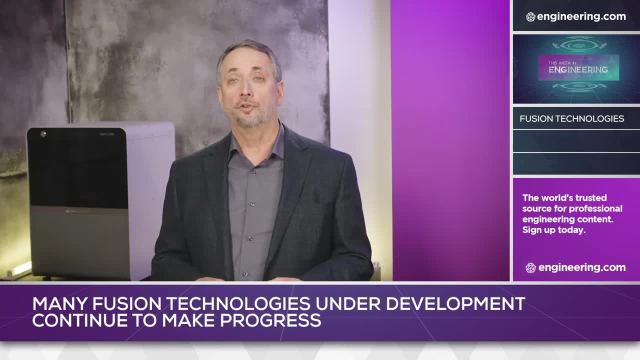 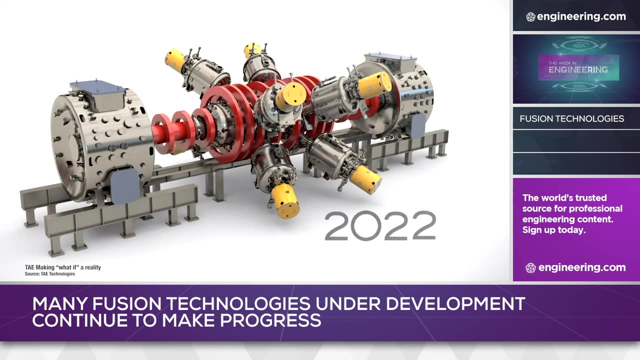 create heat which is absorbed by the liquid metal and can be extracted to power turbines. A test reactor is under construction at a UK Atomic Energy Authority site in Britain. Another novel approach is under development by Foothill Ranch, California-based TAE Technologies, who developed a linear device using technology that the firm calls an Advanced 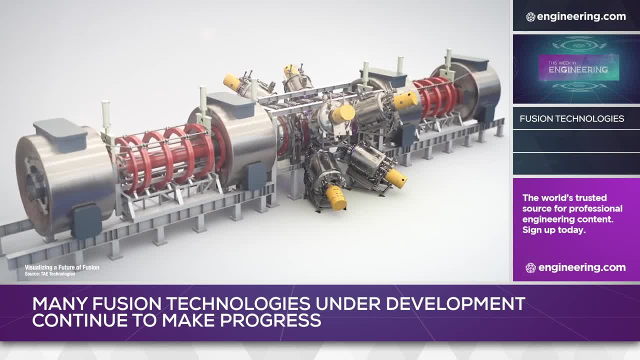 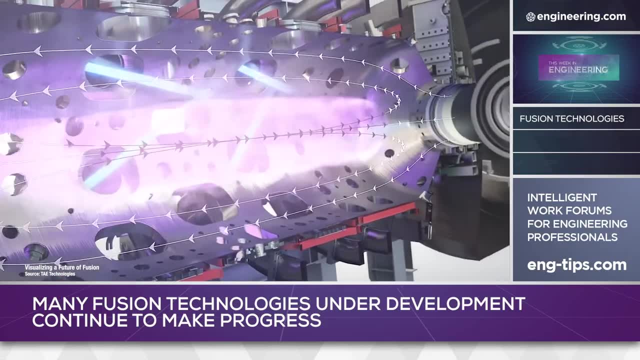 Beam-Driven Field-Reversed Configuration. This approach is radically different from tokamaks or compression technologies combining conventional plasma containment with a particle accelerator in a hybrid arrangement that can accommodate hydrogen-boron, deuterium-tritium or deuterium-helium-3 fuels. 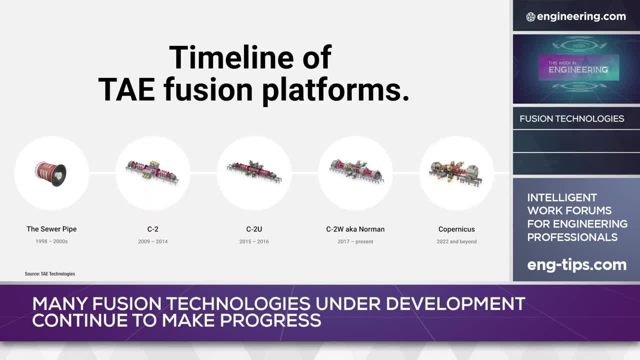 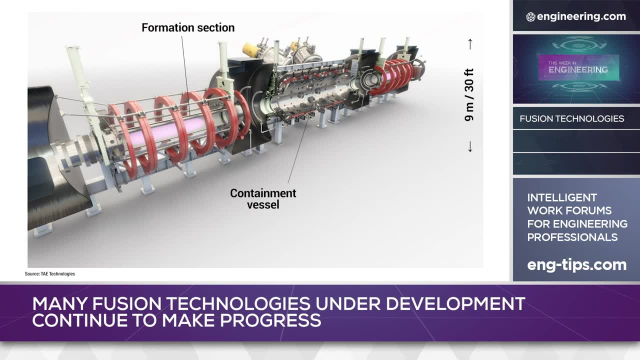 The firm has been experimenting since 1998, and the current fifth generation reactor prototype is compact by large torus standards, at 80 feet long, 22 feet high and weighing approximately 60,000 pounds. The reactor costs £150,000.. 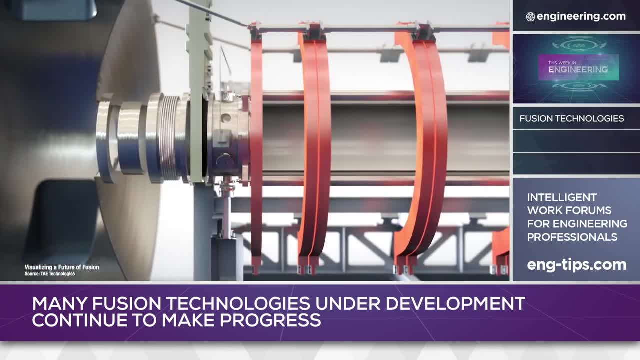 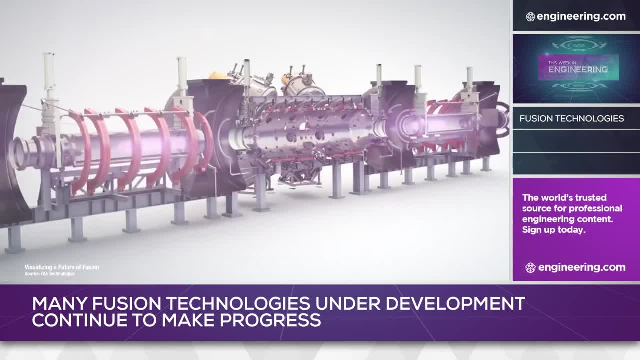 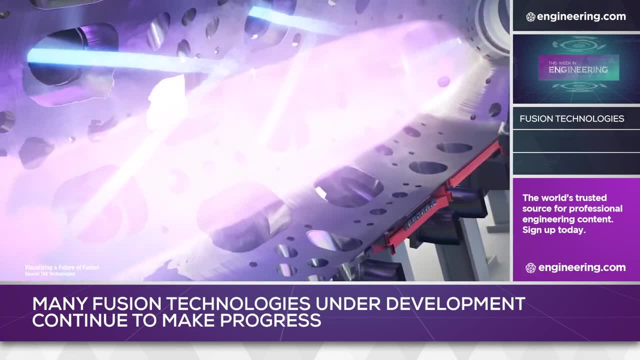 Buel and currently operates on hydrogen and deuterium fuel. The accelerator component of the reactor injects neutral beams to heat and stabilize fusion plasmas, and the firm believes the technology can be adapted to create a treatment system for selectively targeting cancer cells. Power production is, of course, the 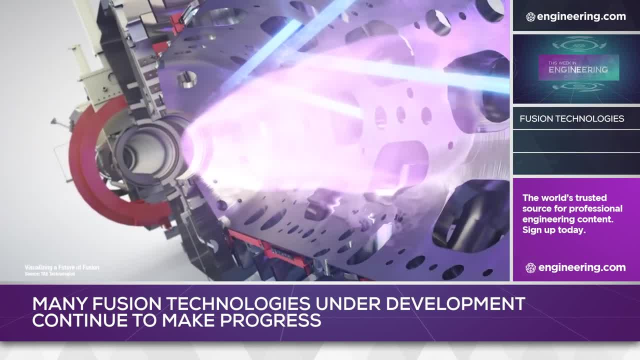 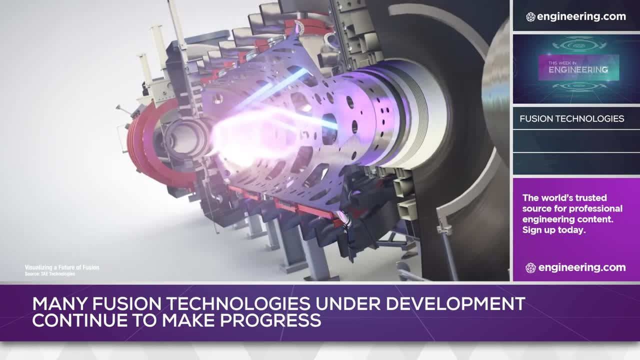 primary goal, and the current system operates at around 70 million degrees Celsius. Temperatures needed for the preferred aneutronic hydrogen boron fuel are several billion degrees, and the temperature rise by a factor of almost 30 will be a technical challenge.